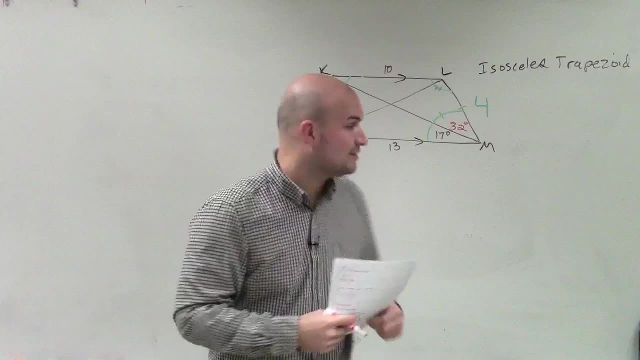 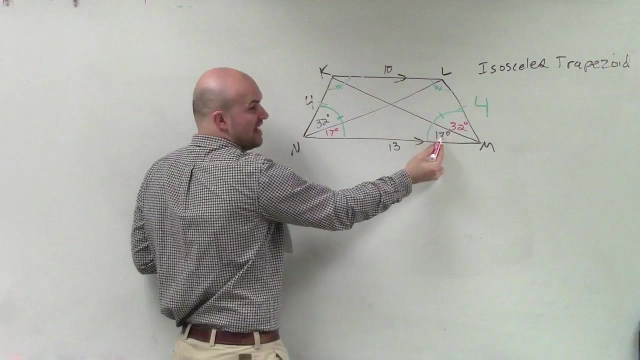 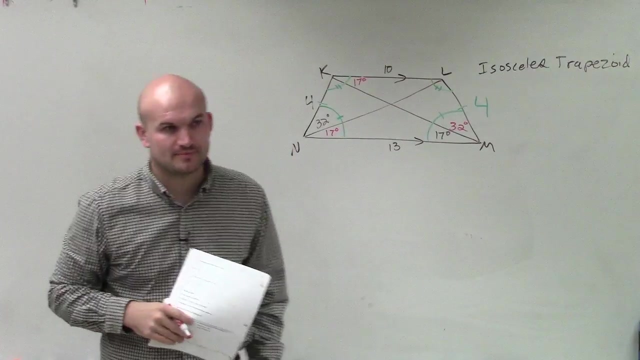 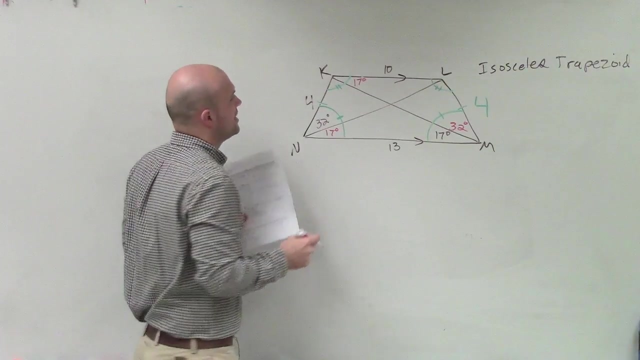 We can also use the idea of alternate interior angles, meaning the fact of, since these are parallel lines, right, and we have this line here, that's a transversal, if that's 17 degrees, by applying alternate interior angles, we know that that's 17 degrees okay, And if that's 17 degrees, then we also know that this is going to be 17 degrees okay. 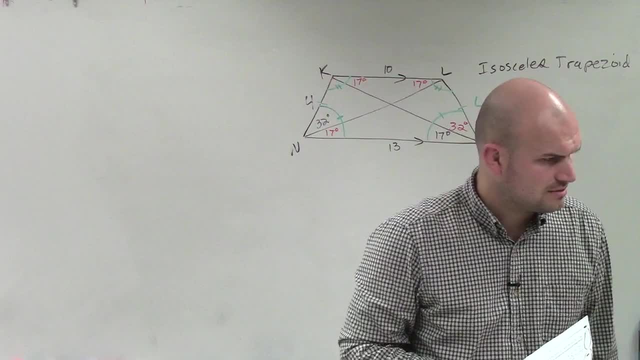 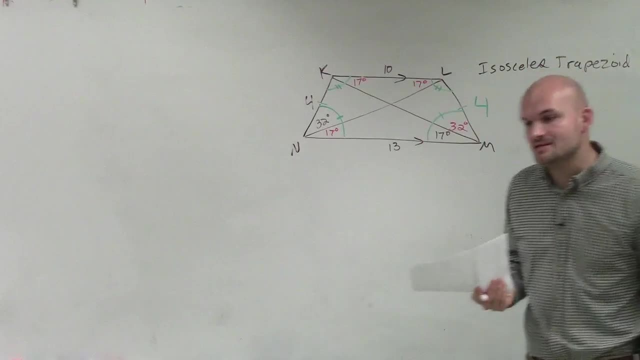 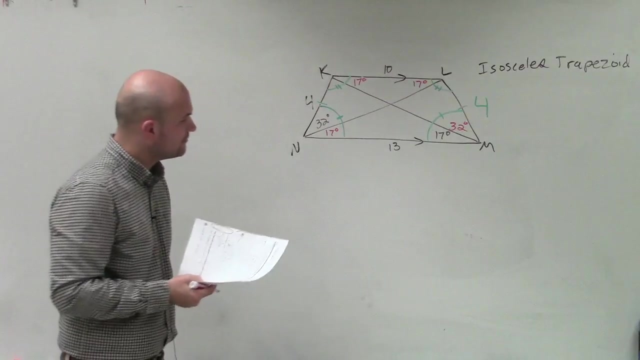 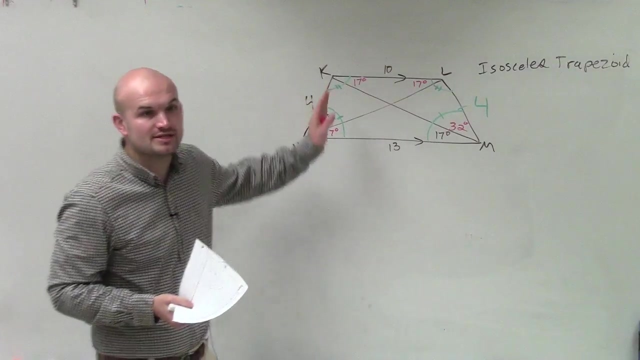 Now another way is to Zach what's wrong. Are you writing this down for me? Now, what was nice about? what was nice about like rectangles, and what was nice about rectangles- and so far we always knew they're, you know, going through to add up to alternate interior sides. 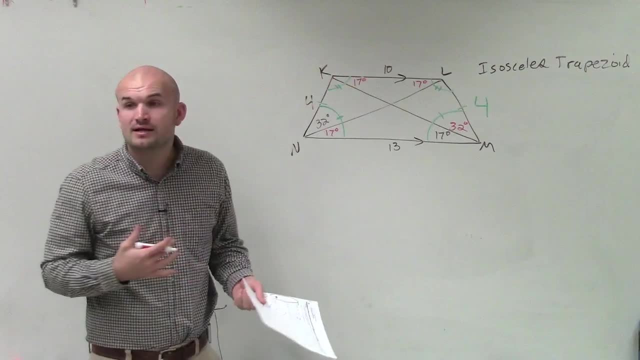 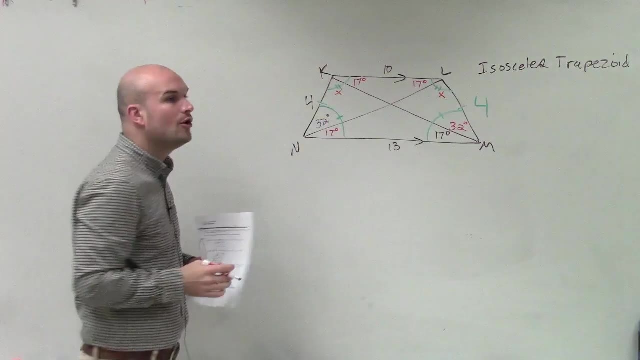 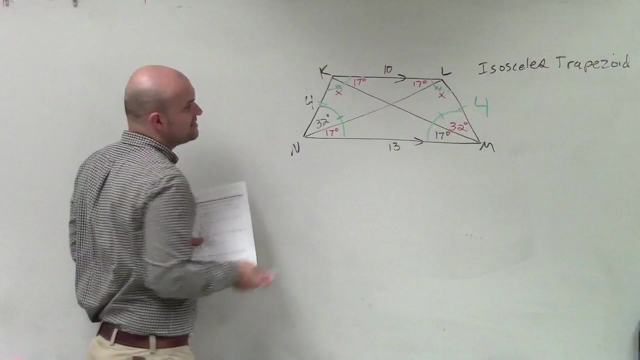 you know that they're going to be on supplementary right. But one thing we notice is, if we look at these two sides, we could say: well, you know what is one thing we know about a quadrilateral, And you don't always have to be thinking about things if we know everything about a quadrilateral. we could say that these two angles 32 and 17 is going to be 49, but what I could say is all these angles are going to add up for a quadrilateral. to how many degrees? How many degrees do we add up for a triangle Which has three sides? 180.. A quadrilateral has four sides, so all the angles add up to 360. 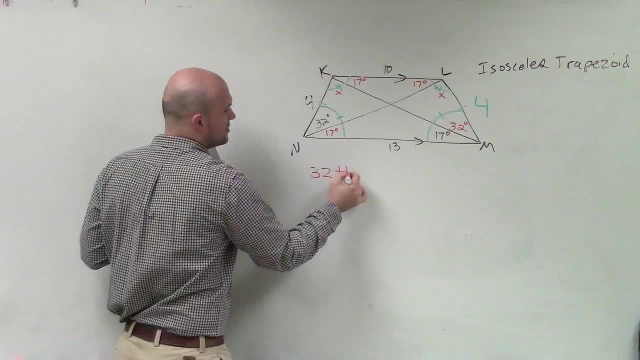 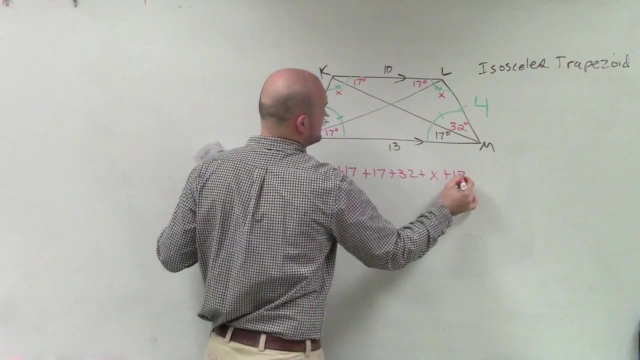 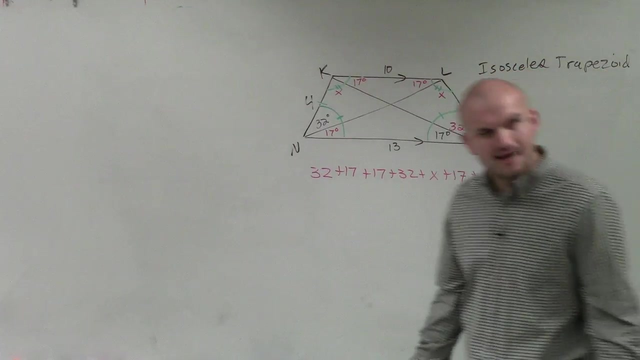 So one thing I could even write guys is: just thinking of it, I could say: 32 plus 17 plus 17 plus 32 plus x plus 17 plus 17 plus x equals 360,. right, You could add up all those. Camille, could you put that face down on your desk please? Thank you. 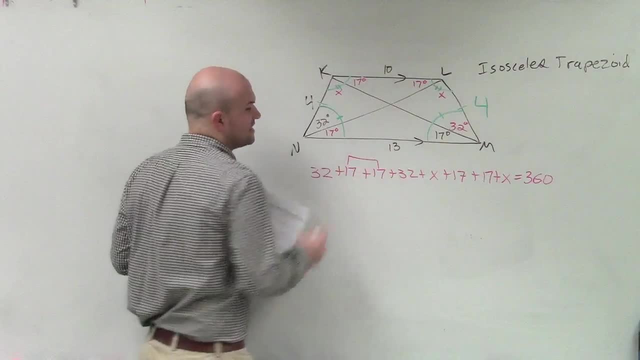 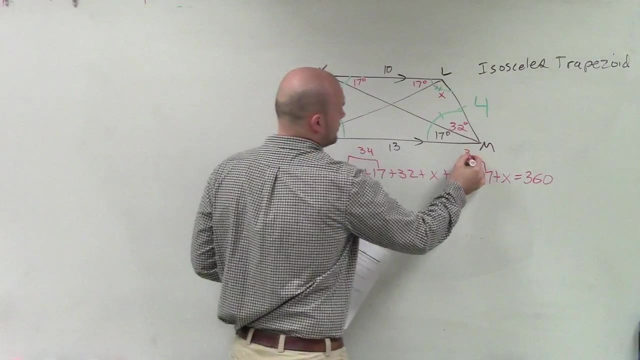 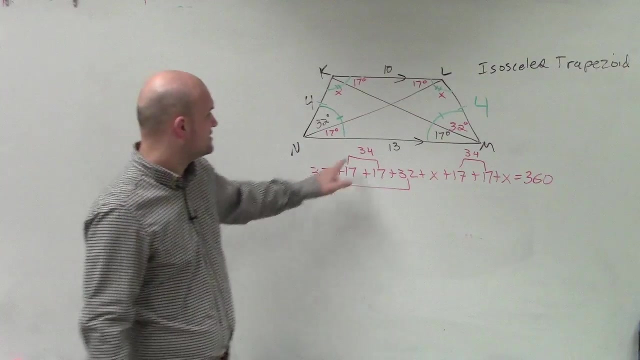 So now, if I kind of add what I have here, 17 plus 17 is 34,, that's 34,. so you could say 34,, 34, and that's going to be 64, so therefore I have 68 plus 64,.